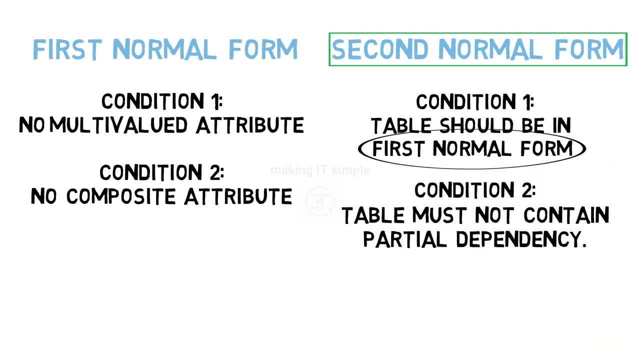 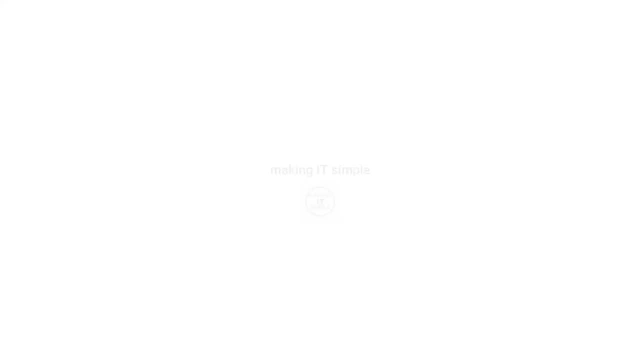 And I have already posted a video on first normal form and also on partial dependency. So I won't go in depth in these concepts But we will see more of examples for better understanding. Let us see both conditions one by one. First condition is table or relation must be in first normal form. 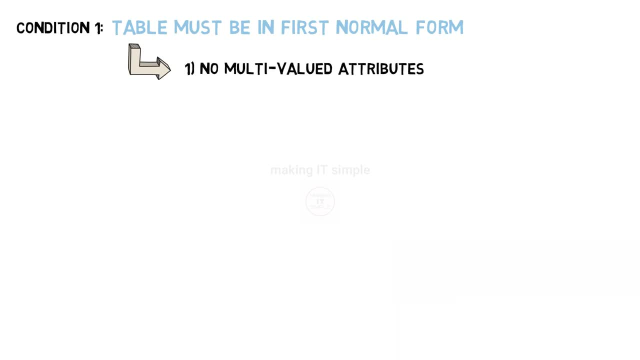 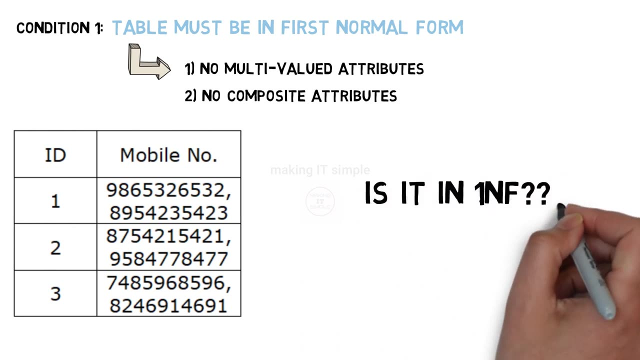 There are two conditions for 1NF: No multivalued attributes and no composite attributes. So if I show you this table and ask whether it is in first normal form or 1NF, what will be the answer? Answer is: it is not in 1NF because this attribute, mobile number, is multivalued. 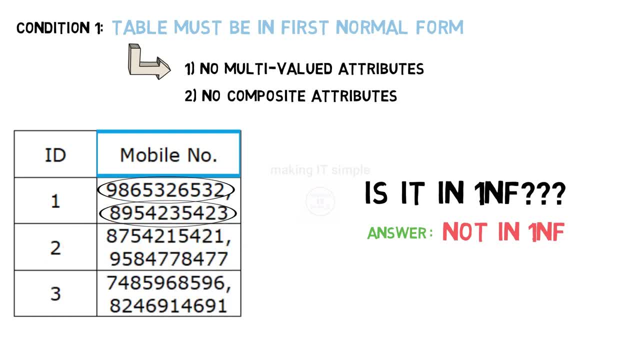 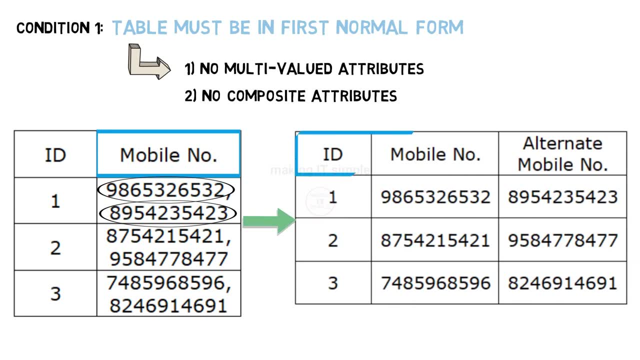 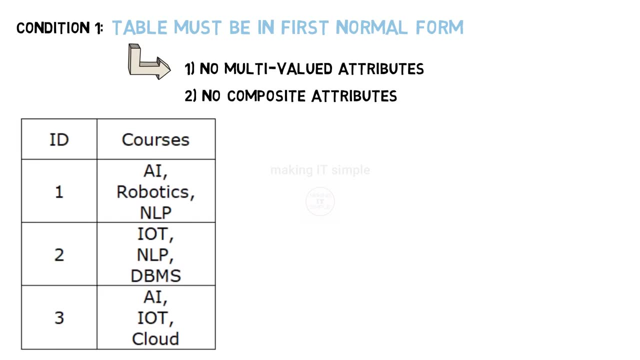 It has two values for each tuple, So it is not in 1NF. If we modify this table into this, then it can be in 1NF, because each column is single valued. Let us take another example. Is this table in 1NF? 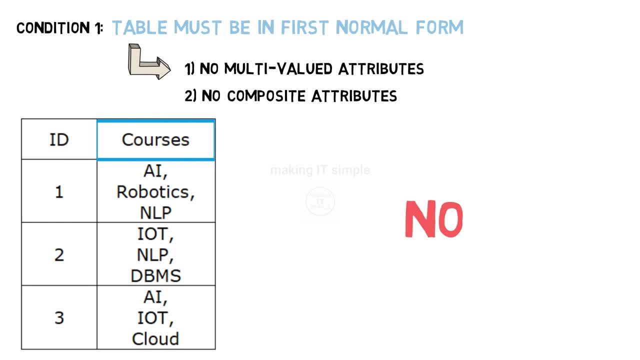 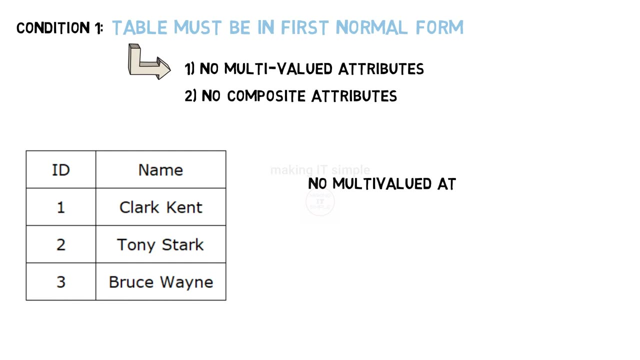 Answer again is no. Courses attribute is multivalued Again. to solve it, we can make these following changes and then we can say it is in 1NF. See this following table. It does not have any multivalued attribute. Is it in 1NF? 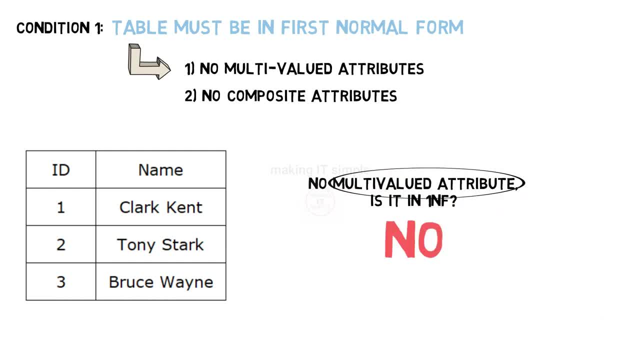 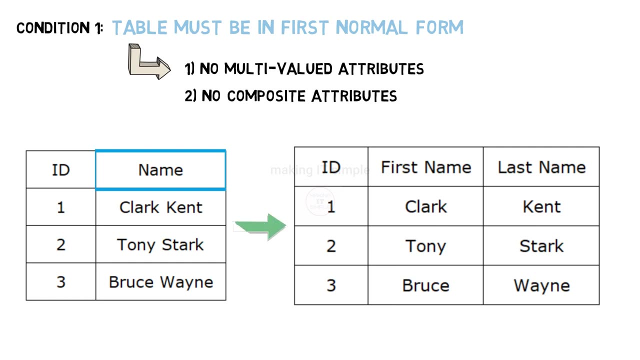 Again, the answer is no. It does not contain multivalued attributes, But it contains attribute name, a composite attribute which can be further divided. So again, this is not in 1NF. We can modify it like this to make it in 1NF. 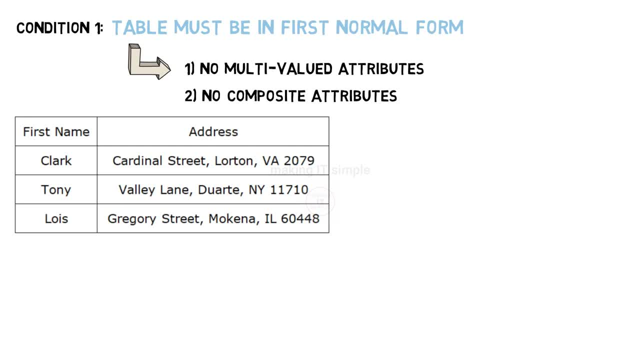 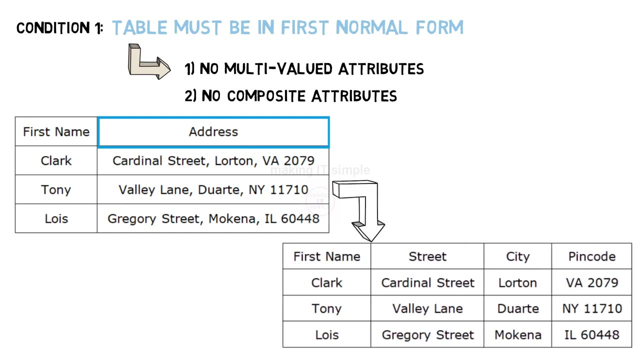 Consider this table and check if it is in 1NF. This also is not in 1NF. You must have guessed it until now. Yes, It contains composite attribute address. To make it into 1NF, we can modify it like this: 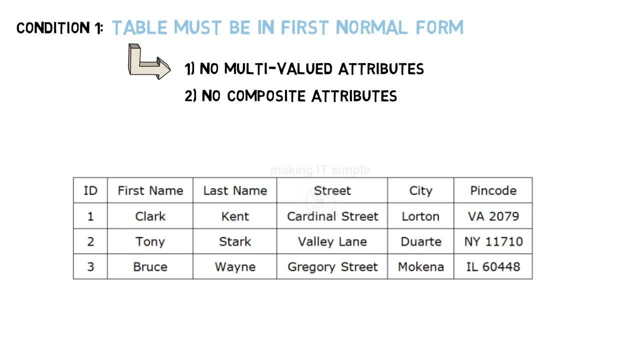 So let us take one last example. This table is in 1NF as it has no composite and no multivalued attributes present in it. So hope you understood the first condition for the table to be in second, normal form. Second condition: It contains composite attribute address. 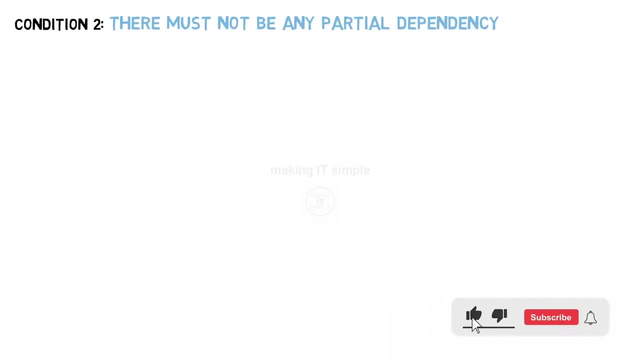 Second condition is there must not be any partial dependency. Let us understand this also with an example. Let us consider this table. To check whether there is partial dependency in a table, first thing you need to identify is candidate key In this table. just by using student id can we identify the complete tuple. 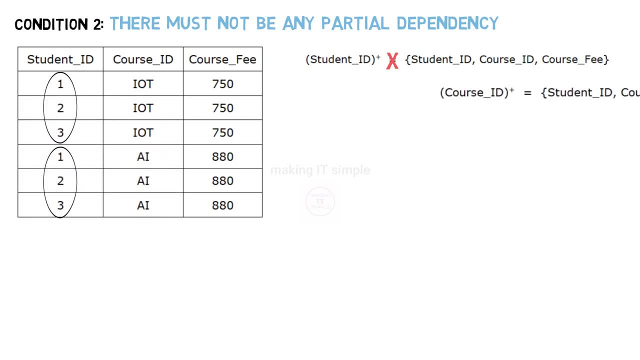 No, There is redundancy present in it. Similarly, In course id we cannot identify complete tuple. It also has redundancies. Same is the condition with course fee. So if you look up closely, by using student id and course id we can identify the complete. 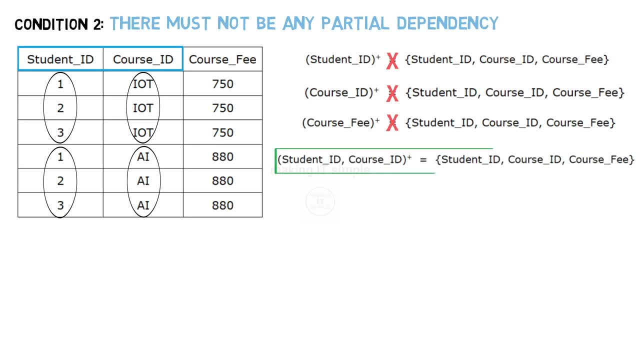 tuple, That is, student id and course id. closure will give us values of all attributes, So we can conclude that student id and course id together form a candidate key. There is only one candidate key in this table. Next step is to differentiate prime attributes and non-prime attributes. 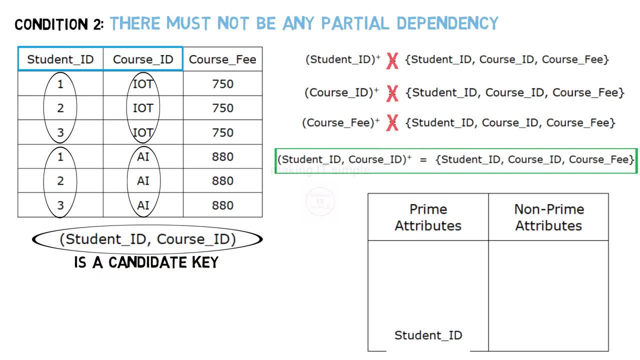 Prime attributes are attributes present in the candidate key, In our case student id and course id. Remaining all attributes which are not part of candidate key or candidate keys are non-prime attributes. In this case, Course fee is a non-prime key. 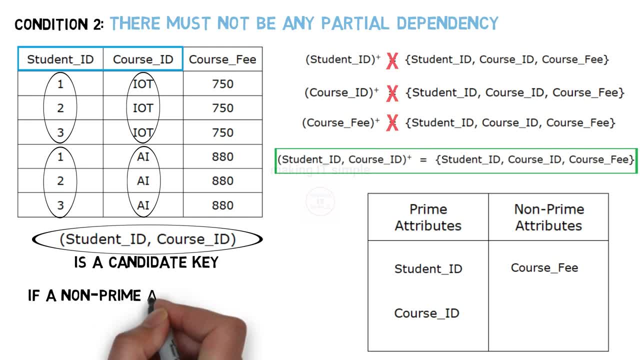 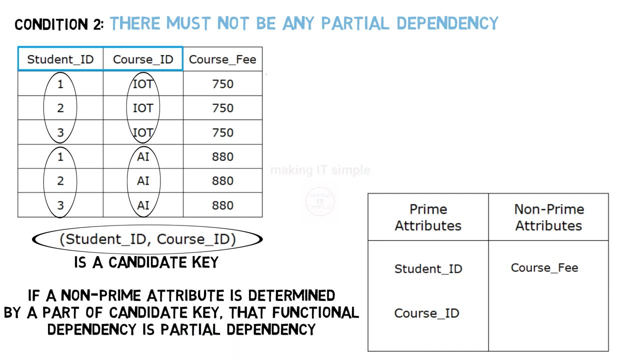 is a non-prime attribute. So partial dependency definition states that if a non-prime attribute is determined by a part of candidate key, that functional dependency is a partial dependency. Let us check student id and course id determines course fee is one of the functional dependencies. 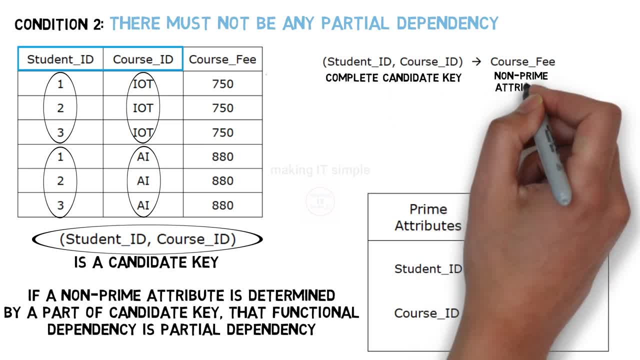 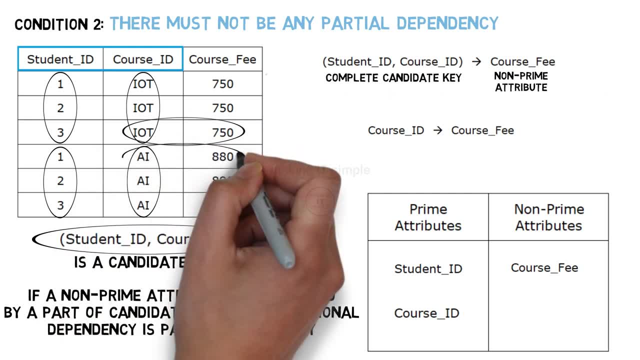 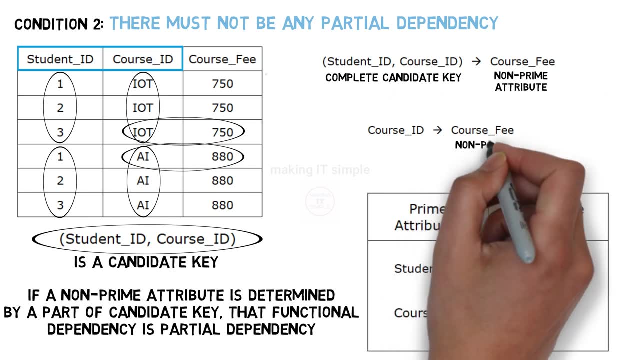 In this case, complete candidate key determines non-prime attribute. Other than that, if you see, by using course id we can uniquely identify course fee, So this can also be a functional dependency. Now, in this case, a non-prime attribute, course fee is determined by part of candidate key.